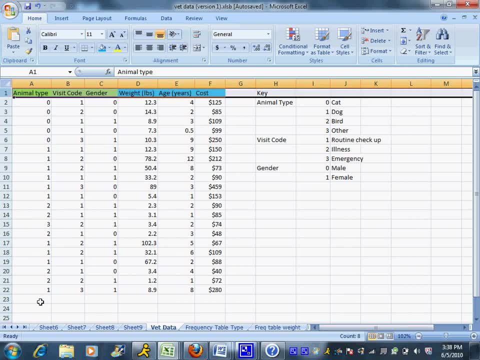 I have to take that out. So I have 21 data points, So that's a good place to start. Now we're going to go through calculating just a few probabilities Maybe, and we can use Excel to help us count these up. So maybe I want to find the probability that a illness is randomly selected. So I'm going to pick an animal and I want to find the probability that they came in for an illness. Well, I can use Excel to count up. 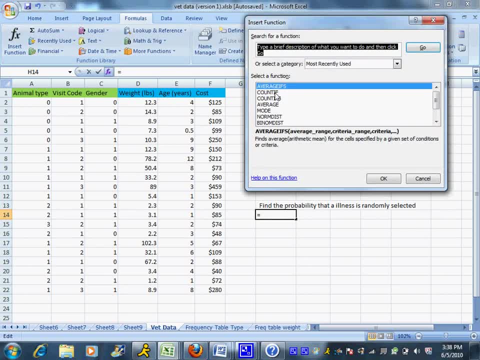 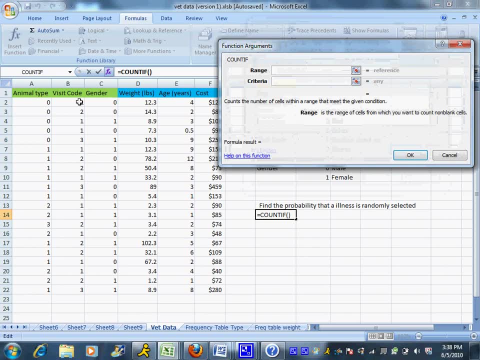 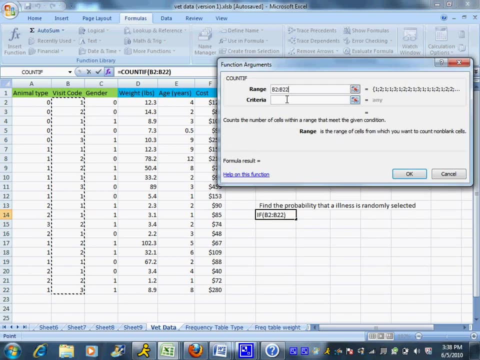 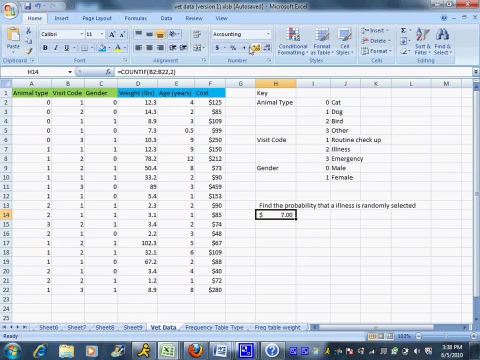 we just talked about this counting how many came in for illnesses So I can use this is just one criteria. So I'm going to use the count, if function, And I want it to count up the visit codes and I want to know how many of those were illnesses. So I have to look and I see illnesses were given the code number two. Now I'll go back and turn this into a number. I turned it into a dollar sign. Now you want to say the probability? 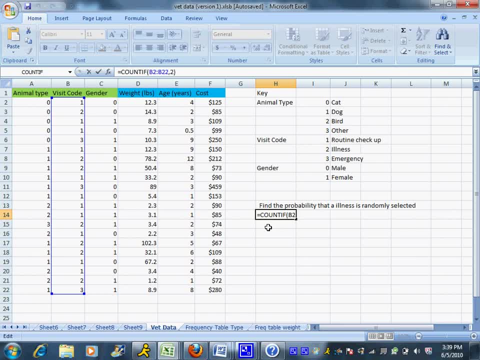 is not seven. Remember I do have to divide by how many I had total. So what I'm going to do is divide this out in the formula bar. I'm going to click on that cell and edit the formula bar. So I'm dividing by 21.. That gives me my probability right there. Now, usually in the business world probabilities are pretty standardly given as a percent. So I'm going to go over to the home tab and click on that percent symbol and the number part of the ribbon and it's going to turn it into a percent for me. Thirty three percent. 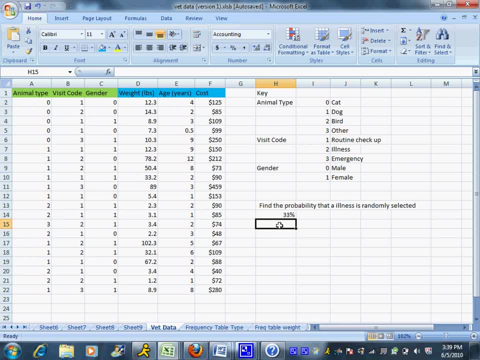 Now, often times when you're calculating probabilities, you might want to narrow it down and look at two things that have to happen. So maybe I want to calculate the probability that an animal, that a dog, came in for an emergency. Now there are two criterias that must be met: that it must be a dog and they must be there. 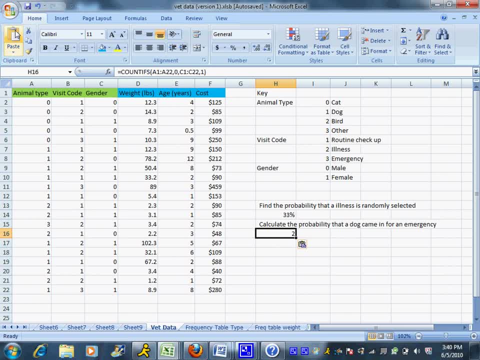 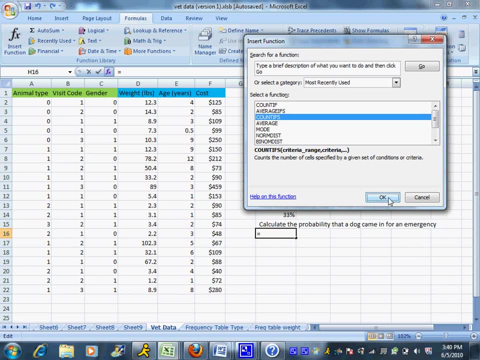 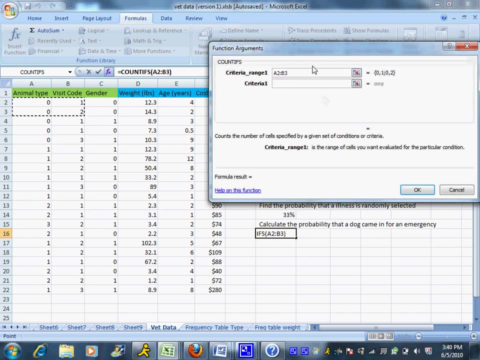 for an emergency, Because there's two criterias. I do want to look at the COUNTIVES function with the S on the end, because it's more than one criteria. So it's got to be a dog. So I'm going to highlight the animal type and I'm going to remember that dogs were given. 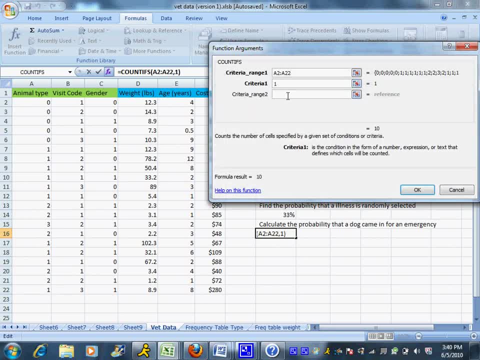 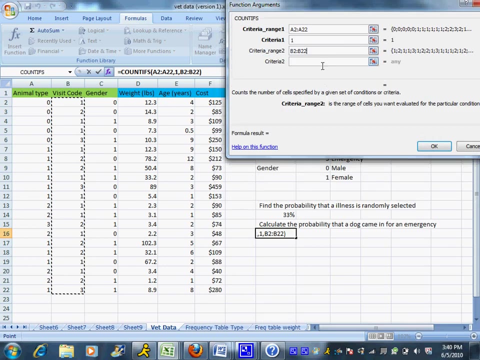 the code of 1.. It came in for an emergency so I'm going to do the visit codes. Okay, Let's make sure it's in the right spot: Visit codes And it's an emergency. so that was given the code of 3.. 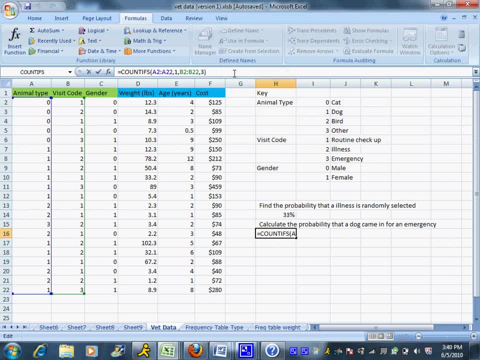 Now again, remember, this is not my probability. This is the number of dogs that came in for an emergency. To calculate it as a probability, I'm just going to divide by 21 and then in the home tab I can turn that into a percent. 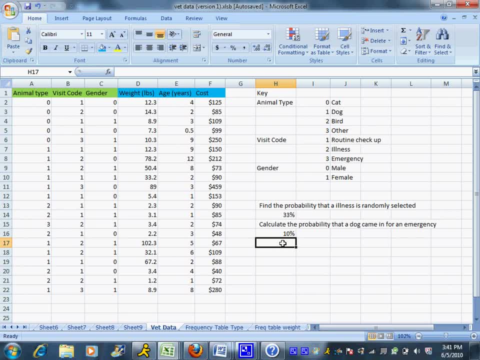 So about 10%. Now the nice thing about the COUNTIVE and the COUNTIVES function is that they are both able to count things given what we call numerical operators, So greater than less than stuff like that. So I'm going to say, calculate a probability that the cost is less than $200. 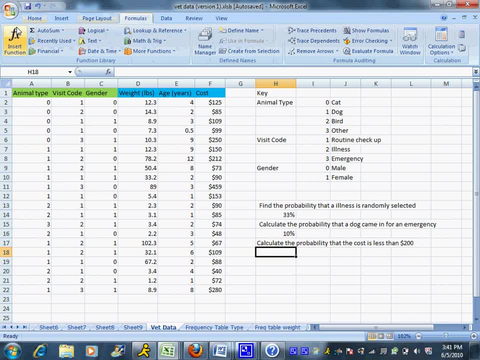 And you don't have to go through and count those up yourself. Excel will do it for you As long as you know what to put in. So I'm going to say: insert a function. This is only one criteria. We're only looking at cost. 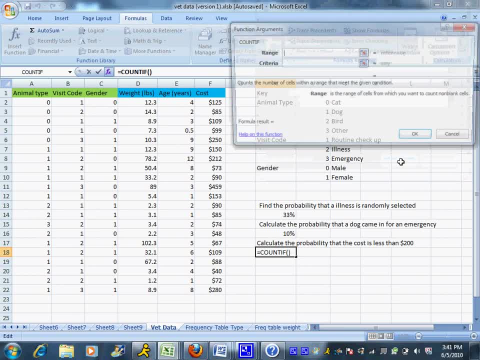 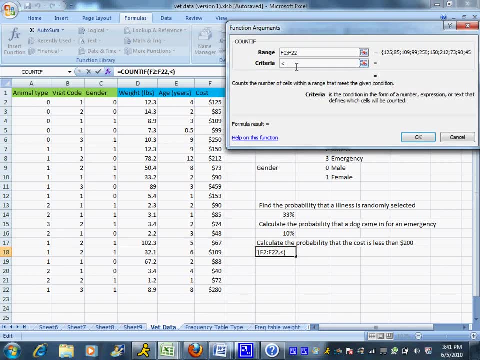 We're not interested in everything else. So I just need the plain old if No S on the end And I'm going to highlight the cost numbers And in the criteria you can use the less than sign Less than $200. 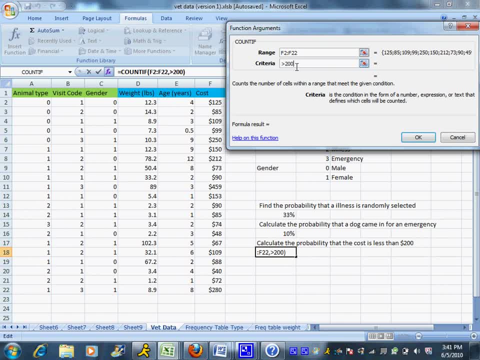 You can also use maybe we're interested in greater than, so that would be the greater than sign, And if you're interested in less than or equal to $200.. I can use the less than and then the equal sign. So I'll do less than or equal to. 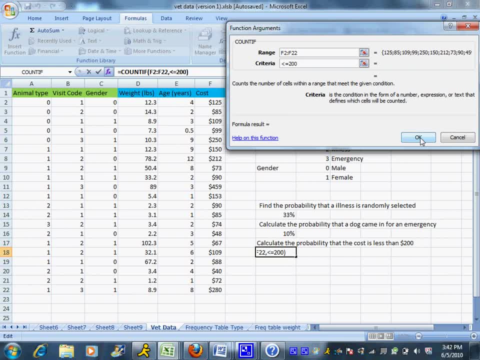 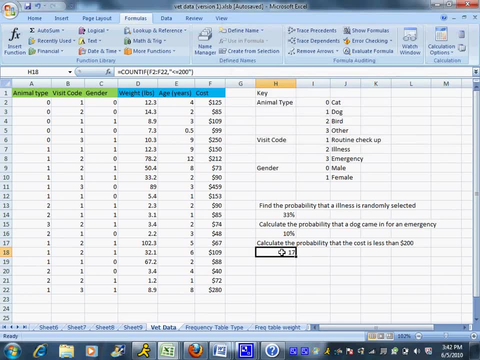 And greater than or equal to works. the same way, You do want to put the less than or greater than symbol first, and then the equal sign. We don't want the equal sign to come first And it's going to say to me: look, 17 people or 17 animals cost less than $200. 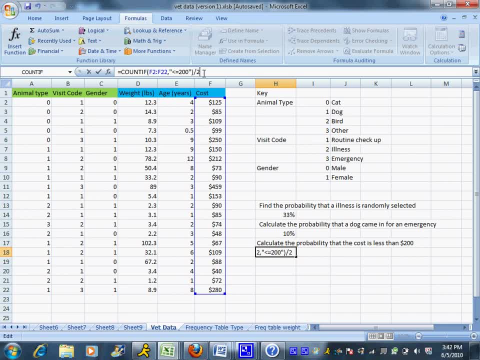 And it's the same idea, not a probability. So I'm going to click on the cell and up on the formula bar I'm just going to type in: divided by the 21.. And I don't want the $200.. So I'm going to click on the cell.